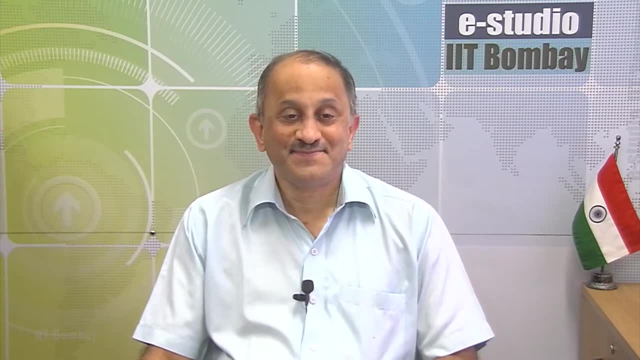 that we shall encounter most frequently. So we are now well set to deal with an example, to understand what we have been learning all this while, And for that example we will take the very same system with which we began our discussion of signals and systems, The. 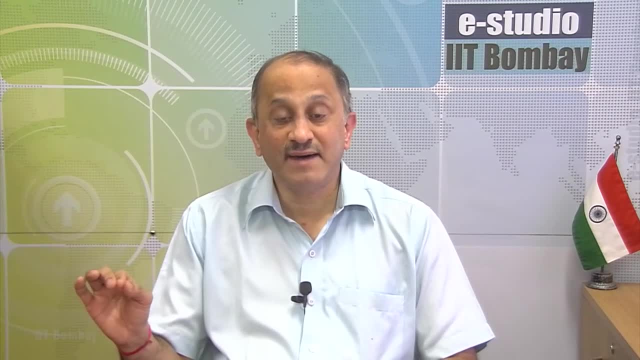 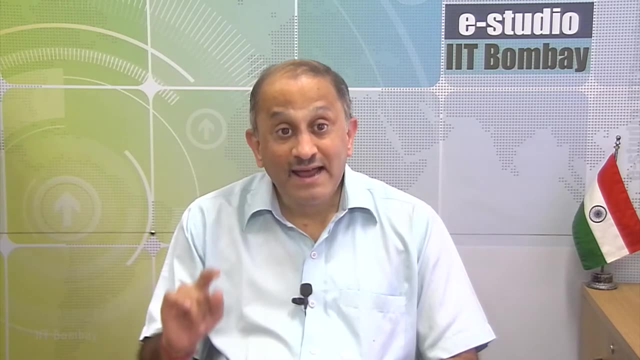 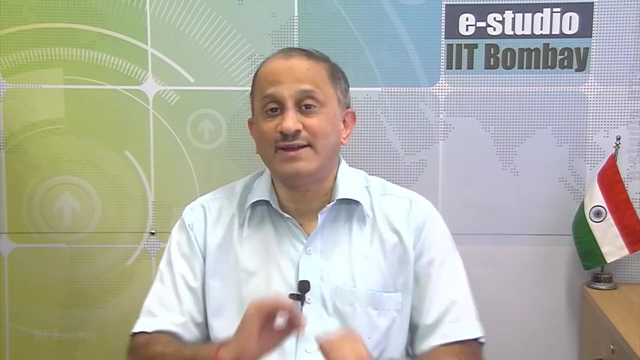 very simple R-C circuit, resistive capacitive circuit, and we would find itself in the same space unit step response using the Laplace transform. You know, it is good to do the same thing in different ways. So you see the connection, and of course then to extend it to other. 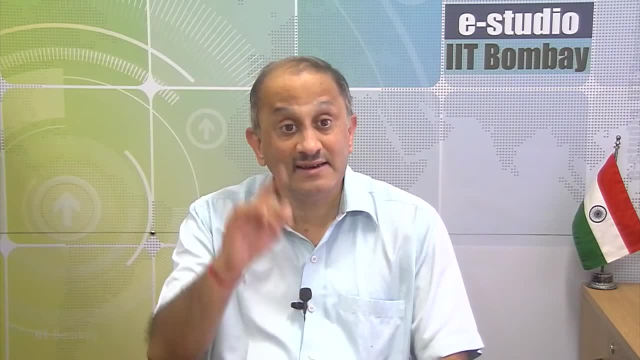 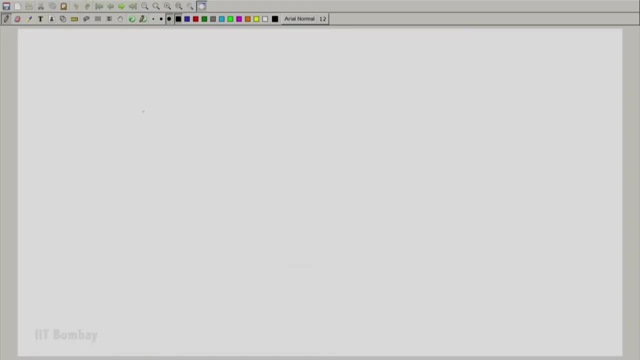 context. So let us do the same thing to the R-C circuit that we did earlier on in module 1, but now use the Laplace transform to affirm our understanding. So here we go, We take this circuit. Now let us write down how each of these 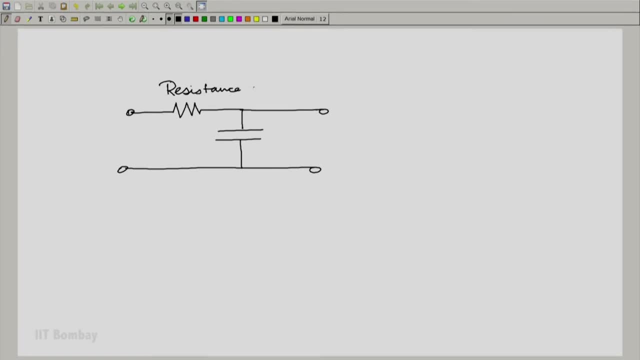 elements behaves. So there is a resistance R and a capacitance of value C And, of course, if you take the individual resistance of value R, look at the voltage across it and the current in it. Then we have V RT. divided by I, RT is equal to R, where upon V RT is equal to I. 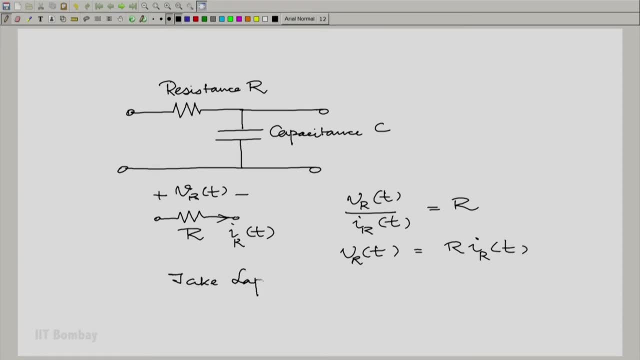 RT times R, And now we can take the Laplace transform on both sides. So therefore, if we take a ratio of the Laplace transform of voltage and current across the resistance, we get just R. It is the same as the resistance, And this quantity, this R, is now also the 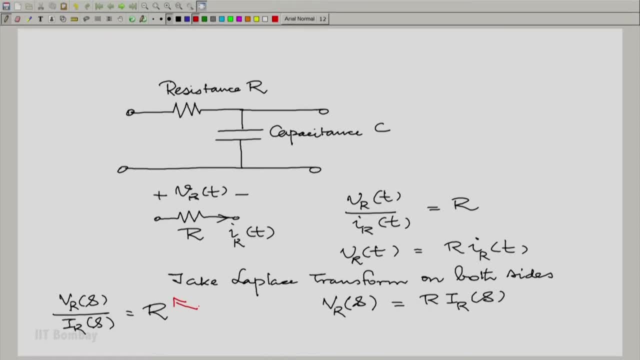 ratio of the Laplace transforms of the voltage to the current, Just as it is the ratio of the voltage to the current, And this is called the Laplace domain impedance of the resistance. In a similar manner, we can take the capacitance and analyze. 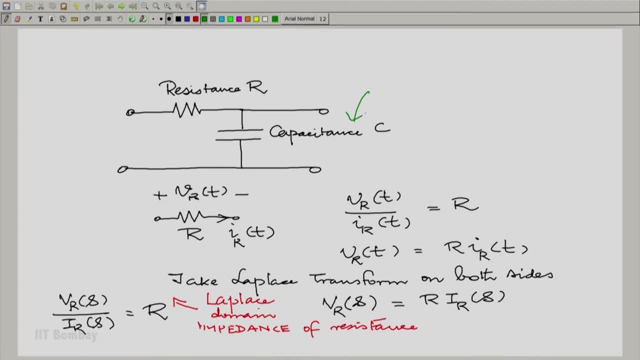 it on the side. So for the capacitance I would have again a voltage and a current associated with it, So V CT and a current I CT flowing across the resistance, So V CT and I CT flowing through it, where upon I CT is equal to C times the derivative of V CT, And we can 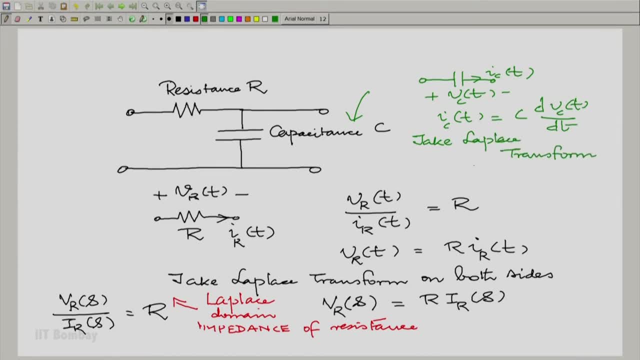 take the Laplace transform on both sides, giving us the Laplace transform of the current is CS. Now remember: when you take a derivative, you are multiplying the Laplace transform by S, So therefore V CS by I CS is equal to C times the derivative of V CT. So this is: 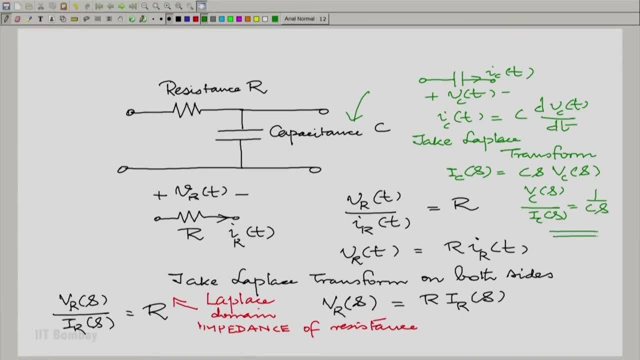 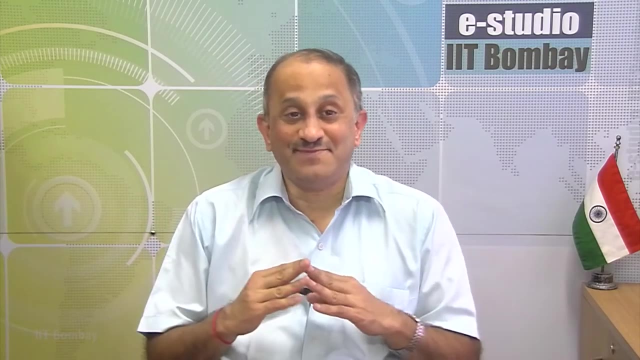 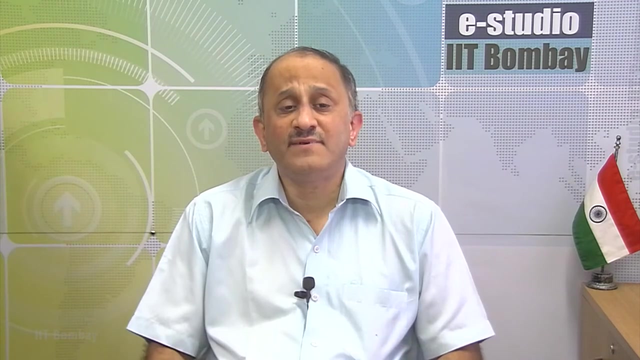 1 by C, S And this now becomes the Laplace domain, impedance of the capacitance. You see, we will study circuits in high school or in pre-college And largely we begin with circuits which have DC excitations, constant voltages. 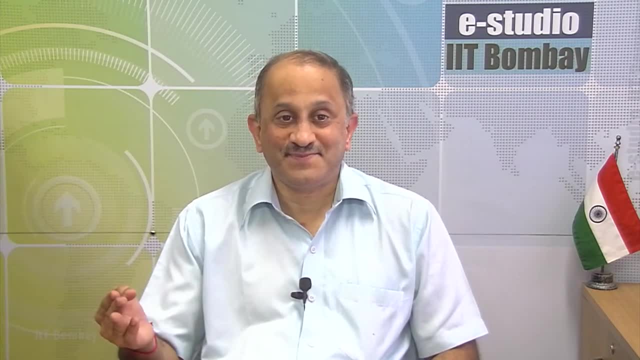 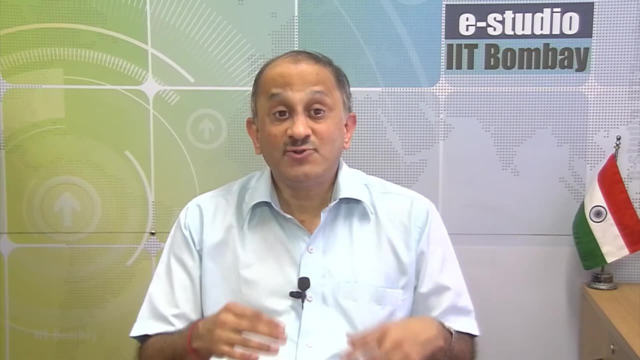 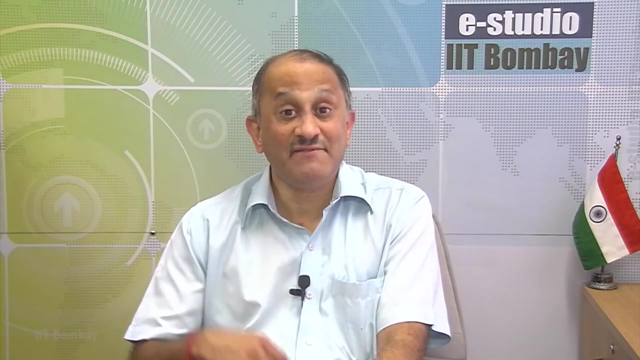 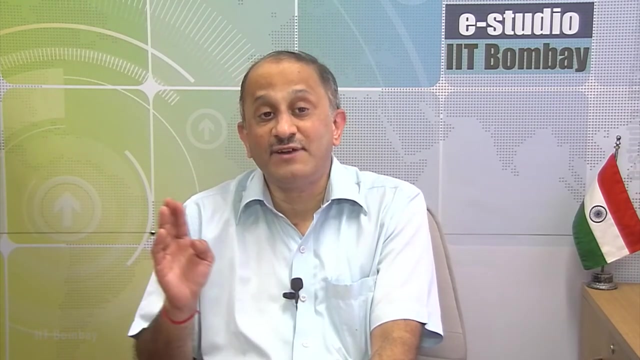 And resistances. So what is often easy to do and convenient to do is to use those principles of circuits carried to other elements as well. So if I have inductances and capacitances, I would like to use the same techniques that I have for resistances and voltages direct. 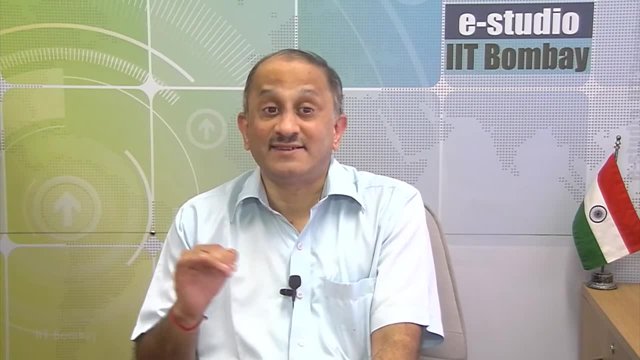 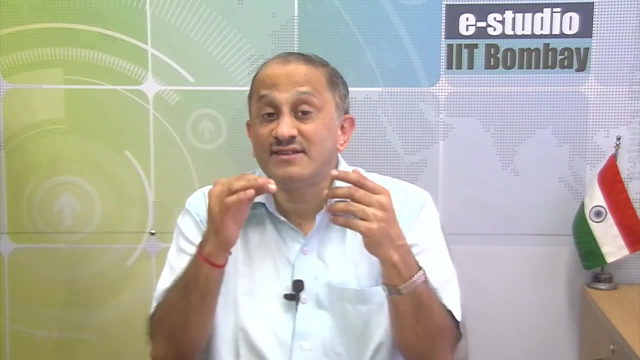 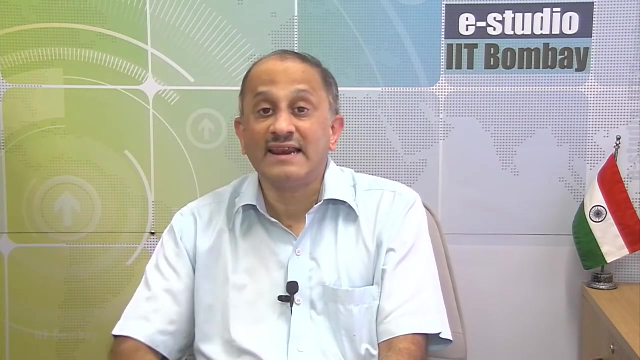 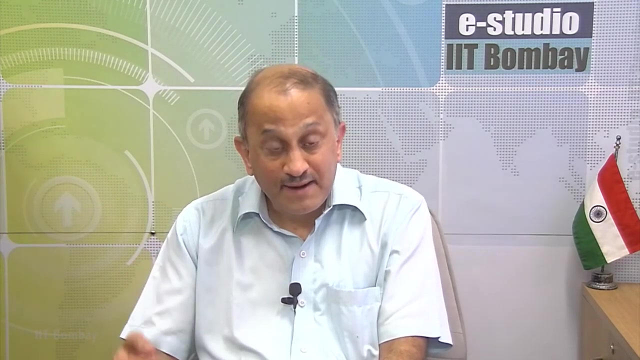 voltages to analyze the circuit And therefore this idea of generalizing the concept of resistance to impedence, Laplace domain impedance, is very useful in analyzing more general circuits than just resistive. In fact, this Laplace domain impedance, together with the Laplace transform of the input and the output can help you handle a much wider class of circuits That can keep coming. 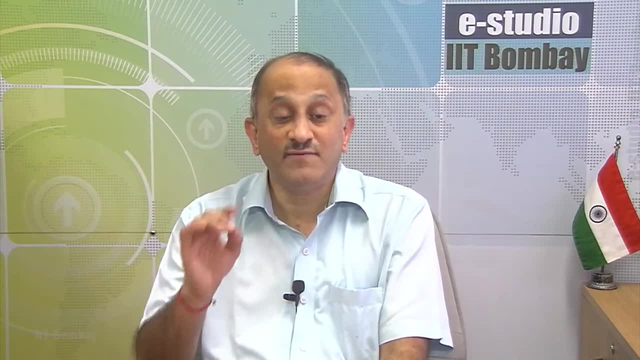 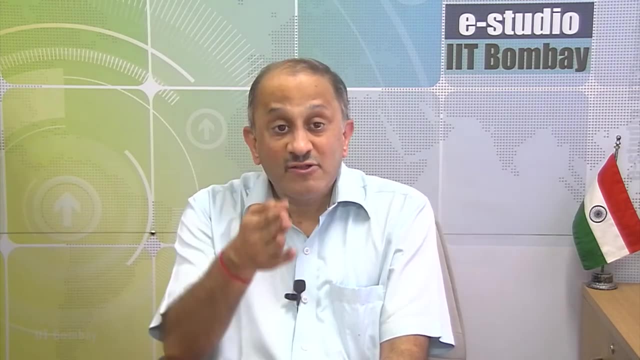 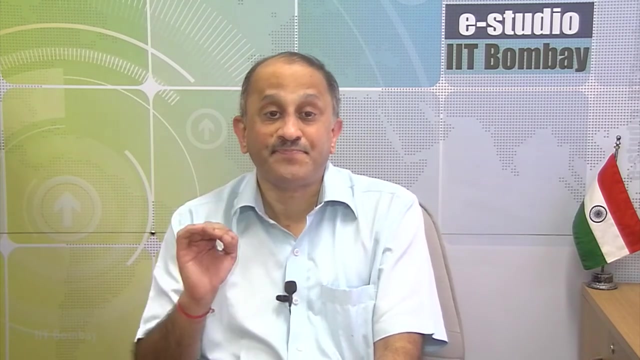 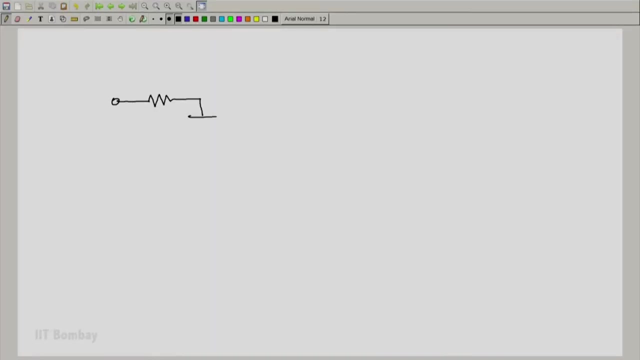 much wider class of circuit situations where you have resistances, inductances, capacitances and sources that could be sinusoidal, starting from a point, or exponential or step or even ramp. Let us now proceed to an example. Let us now draw the circuit again and let us write. 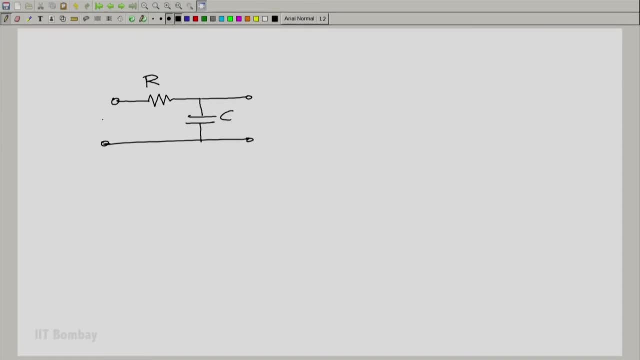 down the input output relationship as we did earlier. So I have input voltage V in t and the output voltage across the capacitor, V out t, and I know the relation between V in t and V out t. We have done that many times before. So there we go. We say V in t is. 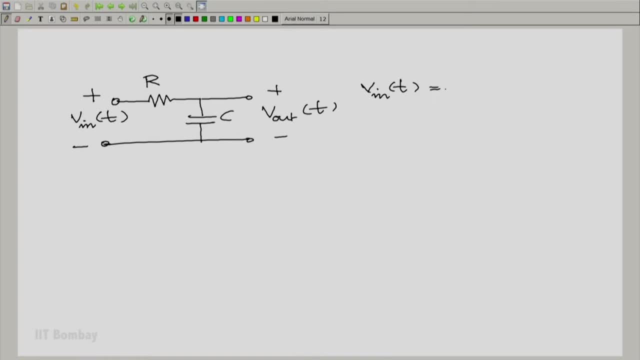 a sum of two voltages. It is the voltage across the resistance, which is R times the current in the resistance. The current in the resistance is the same as the current in the capacitance, which is C times d, V out, t, d, t, and then you have V out t being added to it. So this gives us: 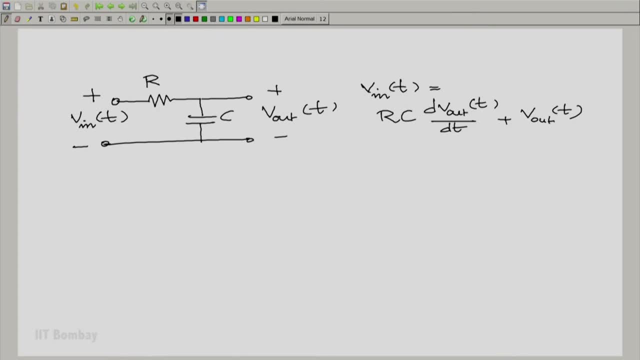 the simple relationship between the input and the output. And now we can take the Laplace transform on both sides. To give V in s Laplace transform of the input is R C s into V out s plus V out s. Essentially here, this is the Laplace transform of the input and this 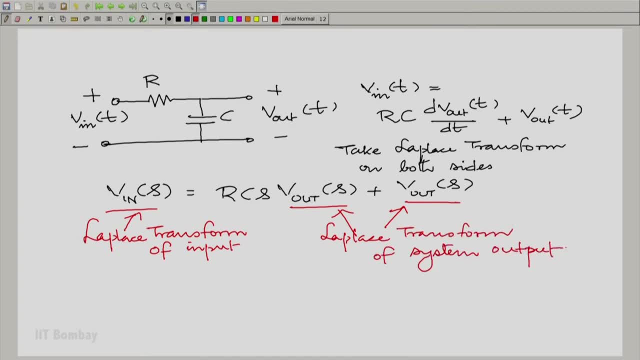 is the Laplace transform of the output, And we have a system here. The system is the R C circuit And we can now write down the ratio V out s by V in s, which is 1 by V in s. So 1 by 1 plus R C s. Let us put R C equal to the time constant tau, So we get 1 by 1 plus. 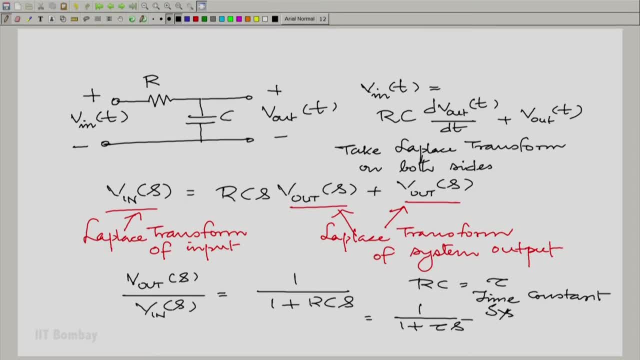 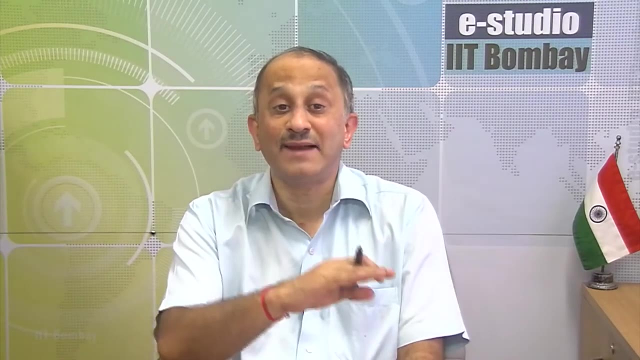 tau s. This is the system function of this system, simple example of system function. And now, of course, we can find the impulse response. very easily, We can find the impulse response by inverting the Laplace transform. Now, of course, here is the Laplace transform. 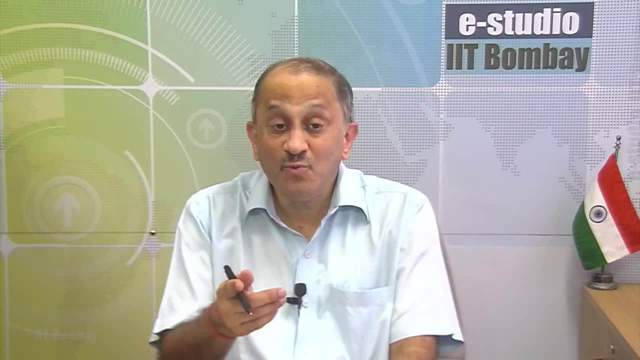 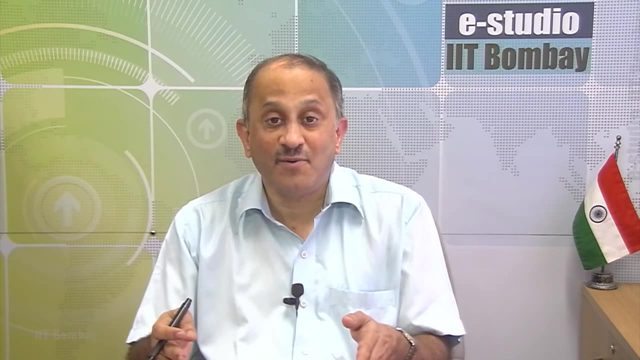 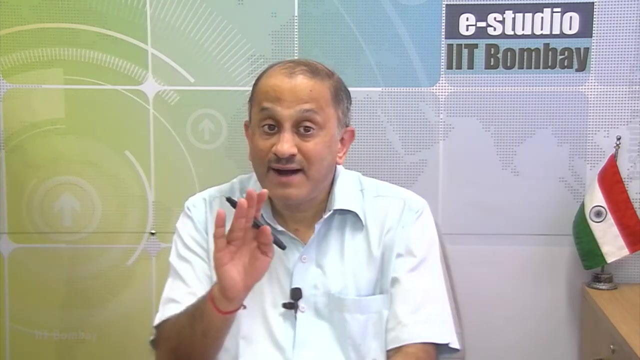 Here it is very easy to invert, because you know which region of convergence to choose. You see, when you have a rational Laplace transform, all that you have to remember is that the poles of the Laplace transform cannot be a part of the region of convergence. So 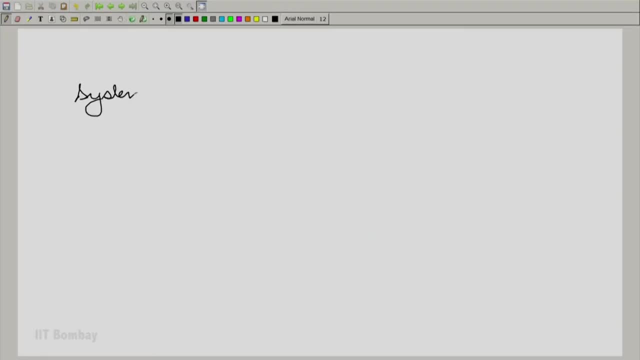 here. in this case we have only one pole. So in the s plane the pole is the original, is at minus 1 by tau on the negative real axis And therefore there are only two possible regions of convergence. You see, as I was saying, the Laplace transform, if you have. 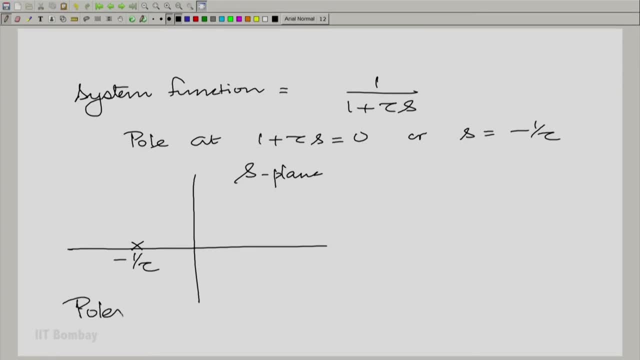 a rational Laplace transform. the poles need to be excluded from the regions of convergence And therefore you can have two possible regions of convergence here. Let us mark them, draw a vertical line through this pole And the right shaded region is one of the regions. 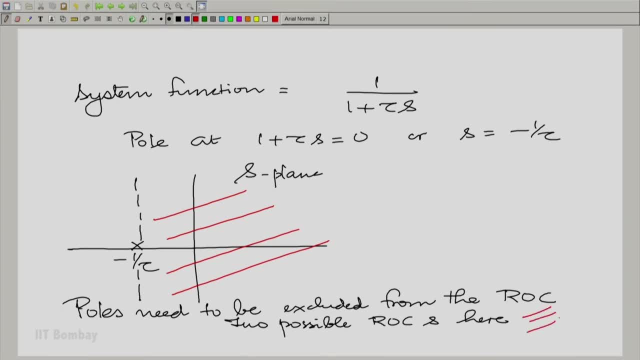 of convergence. I will mark that here, And the green left shaded region is the other possible region of convergence. Now, this would give us the right sided impulse response And this would give us the other one, would give us the left sided impulse response. But 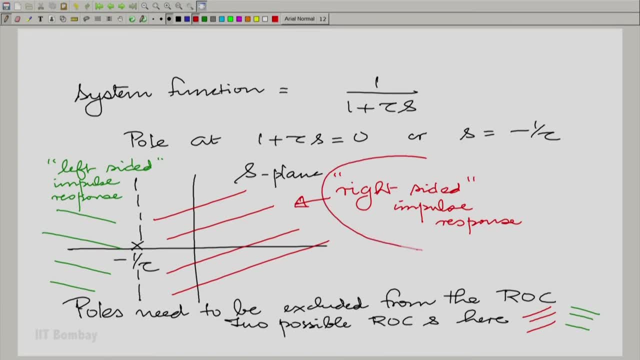 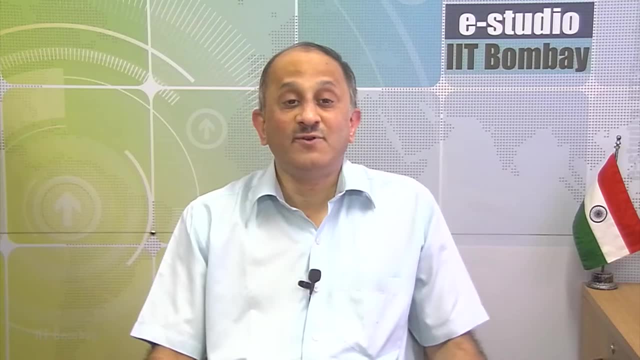 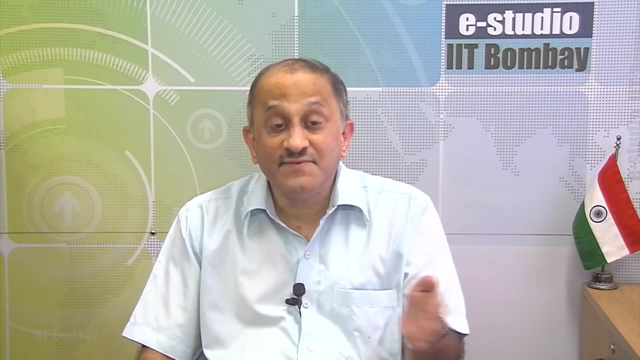 we have to choose the right sided impulse response. This has to be chosen on account of causality. You will remember that if you want the system to be causal, its impulse response needs to be 0 for all negative t, And that is only possible if the signal is. 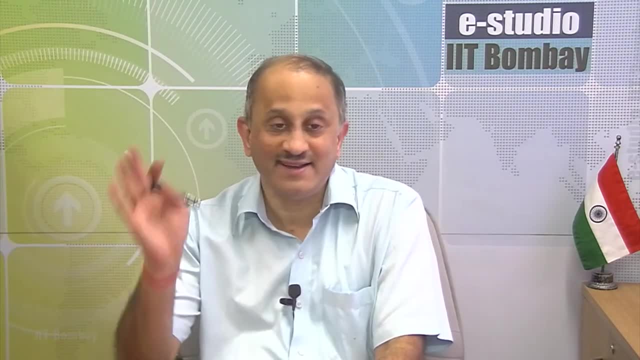 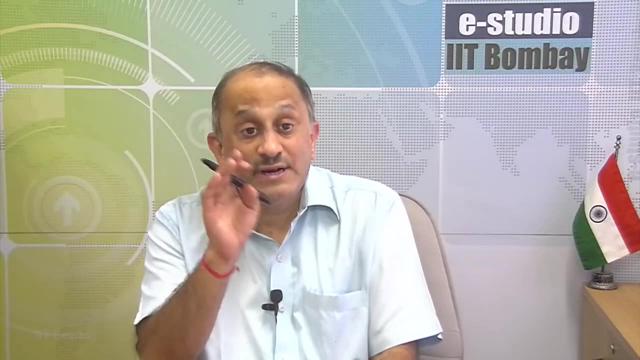 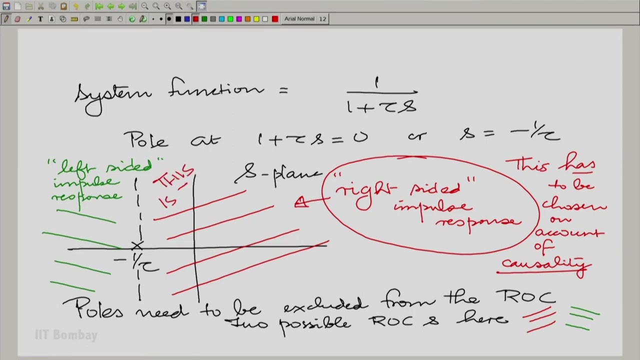 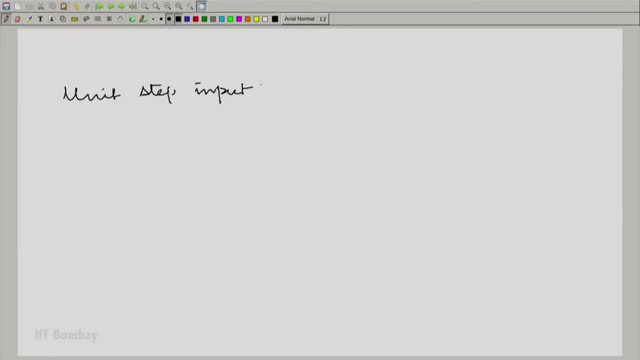 right sided. So we have a very clear choice to make here Now. having chosen that let us give a unit step input to this system, So we have this. This is the system function here. We have made this choice. This is the ROC now, And let us give it a unit step input. That means: 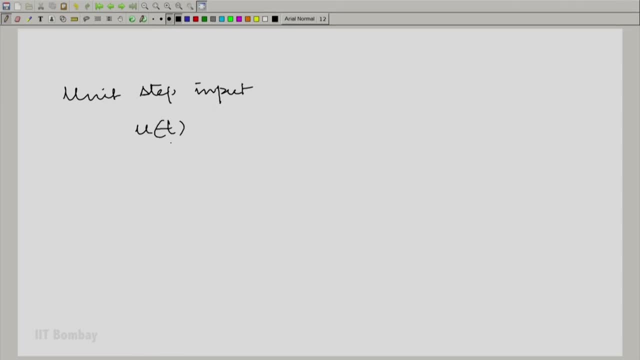 we are giving it ut as the input and the Laplace transform of ut is equal to 0. And this is of U. t is very simple. Now, of course, here we need to worry about the region of convergence, and the region of convergence is going to be real part of S greater than 0. And for 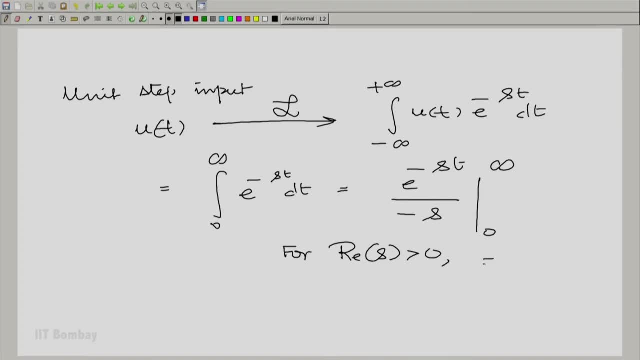 real part of S greater than 0, this becomes essentially 1 by S. So this is the region of convergence and this is the expression of the Laplace transform. And if we give this input, that means if we make V in S equal to 1 by S, then V out S is going to be V in. 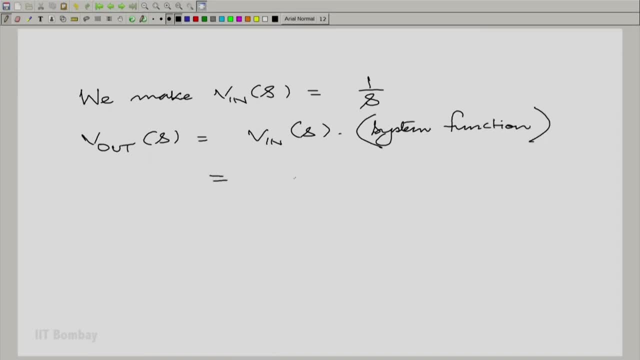 S times the system function and that is 1 by S times the system function And I can make a partial fraction expression. To make a partial fraction expansion, it is easier for us to write it in the form that we know, the standard form. So: divide numerator and denominator by tau, 1 by tau into 1 divided. 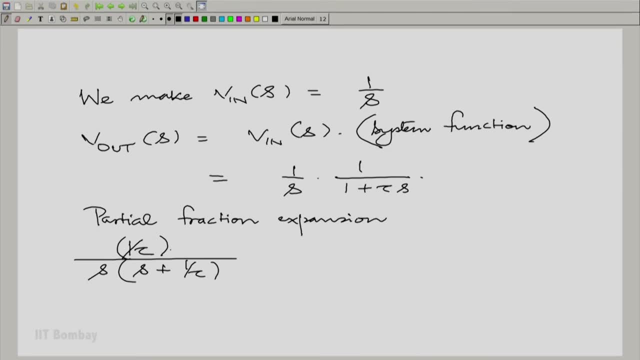 by S into S plus 1 by tau, And this can be expanded as something divided by S plus something divided by 1 or something divided by 1. Something divided by S plus 1 by tau. And to get this we multiply by S and put S equal. 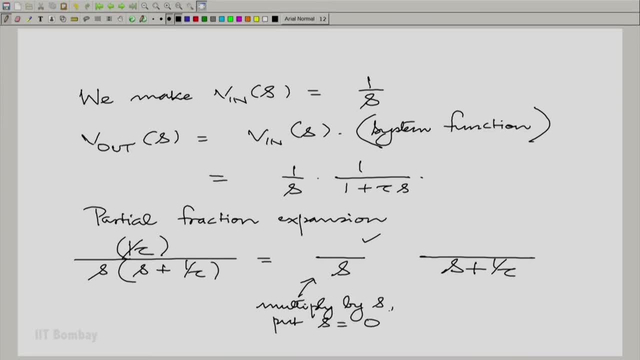 to 0, whereupon we would have 1.. And to get this, we multiply by 1, or rather just S plus 1, by tau, and put it equal to 0, and that gives you minus 1.. And you can of course verify that this, indeed the right hand side, indeed sums to the left. 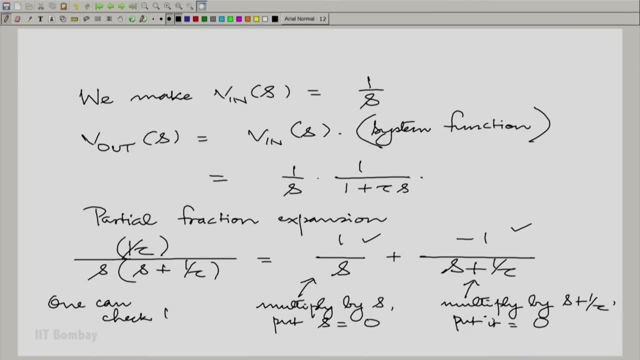 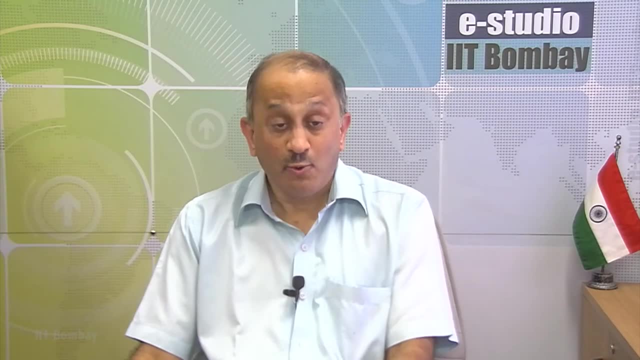 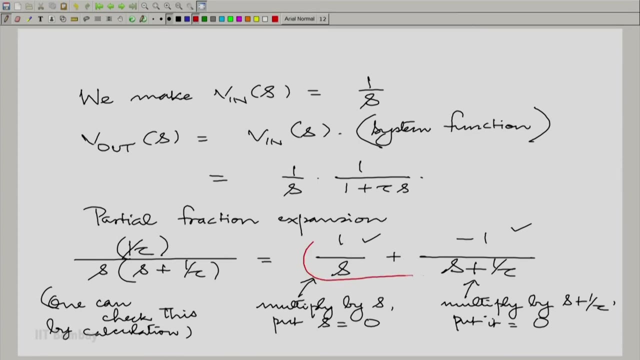 hand side. That is not very difficult to do, So one can check. It is always a good idea to check your partial fraction decomposition. What I mean by check is here, for example, let us see. You see, I can simply aggregate this, This can be aggregated, So this is. 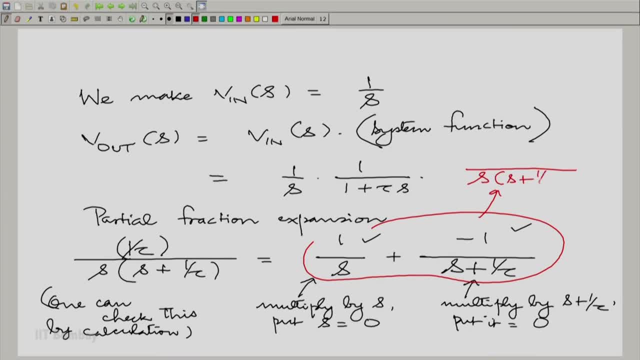 S into S plus 1 by tau S plus 1 by tau minus S, and that is indeed equal to the left hand side. So, checked, It is always a good idea to do that if you are not sure. So now we. 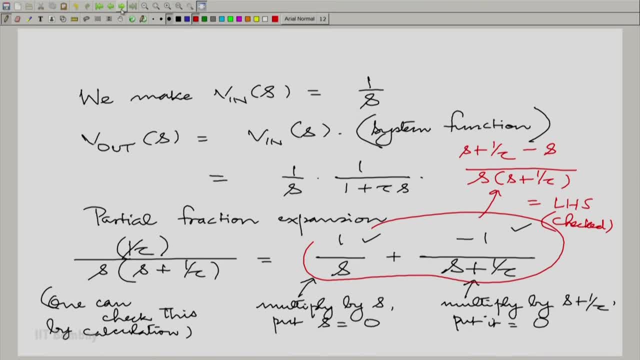 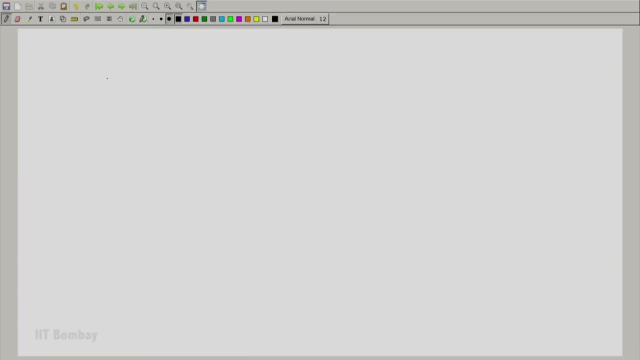 have this partial fraction, expansion, and we need to recognize the regions of convergence. What regions of convergence, What regions of convergence do we have to associate? So, essentially, V out S now is 1 by S minus 1 by S plus 1 by tau, and this came with the ROC, real part of S greater. 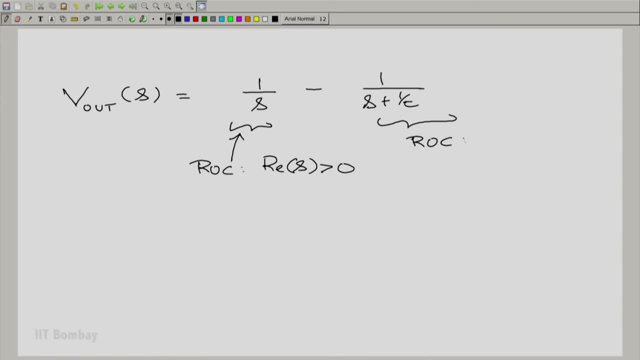 than 0.. This came with the ROC real part of S greater than 0.. So we have this partial fraction is greater than minus 1 by tau, and the only way in which we can reconcile these ROCs is to take their intersection. The intersection which is real part of S greater than 0 must. 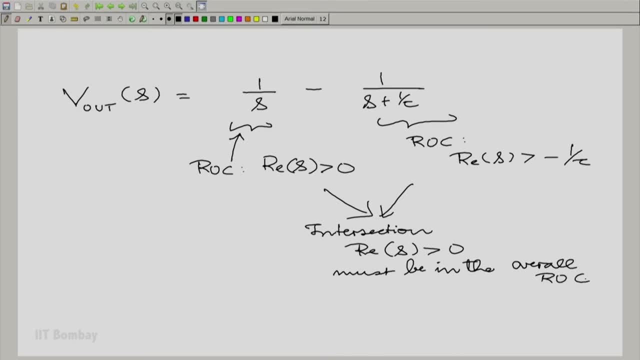 be in the ROC and we can use that to invert this. And when we use that to invert we get V out t. very simple is u t, that is the inverse of 1 by S minus e raise to the power minus t by tau times u t, or 1 minus e- raise to the power minus t by tau times u t, which is indeed. 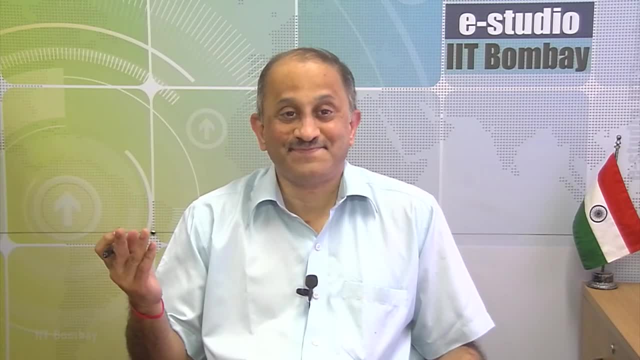 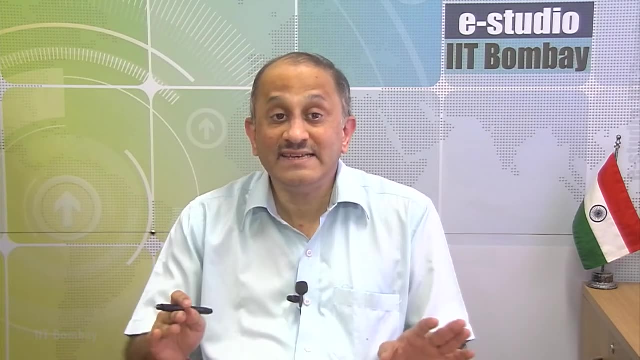 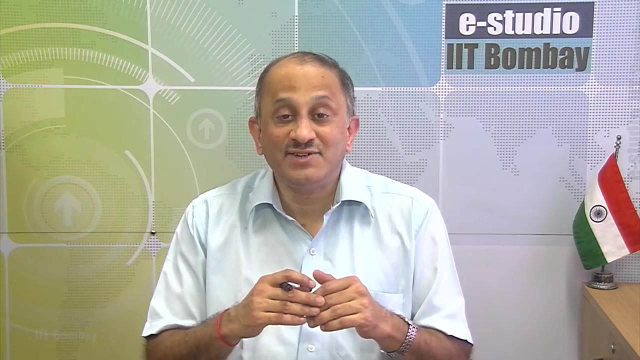 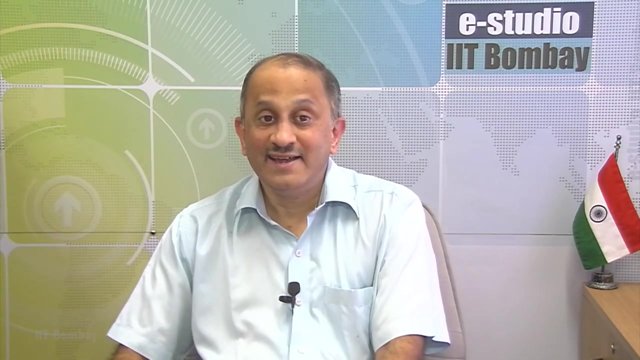 the step response that we had got much earlier. Simple and elegant. Laplace transform is a simple, neat, algebraic way, using algebra first, just plain, you know, addition, multiplication and finally the experience of inverting a rational Laplace transform. Now it would. 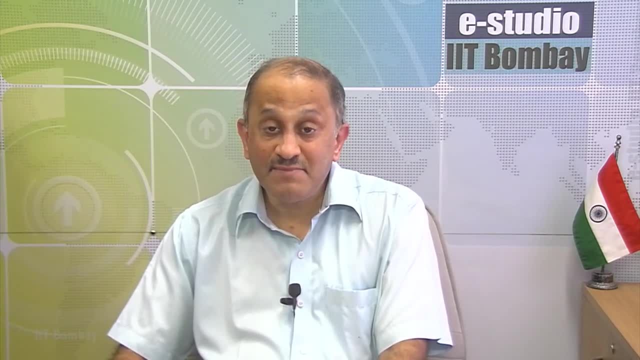 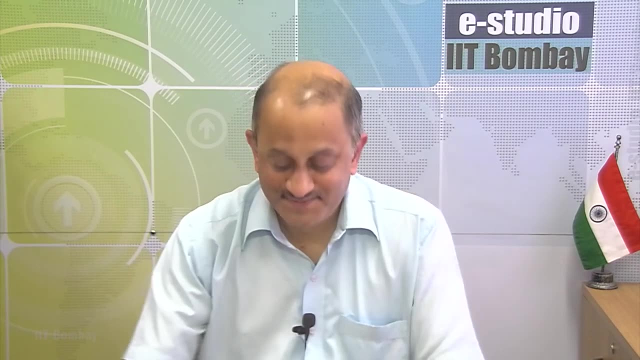 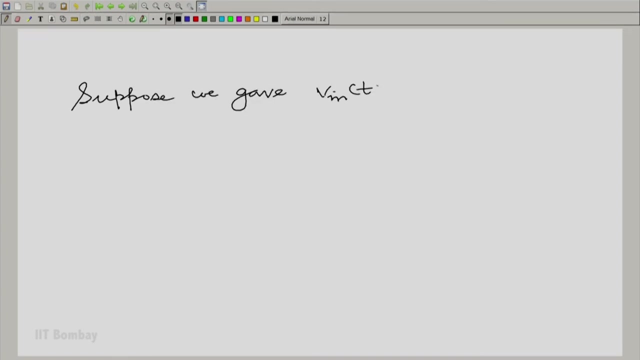 be interesting to see what happens if you gave the same circuit not a unit step but a unit ramp. So let me explain what I mean by that. Suppose we gave this a unit ramp input now Essentially an input that looks like this: 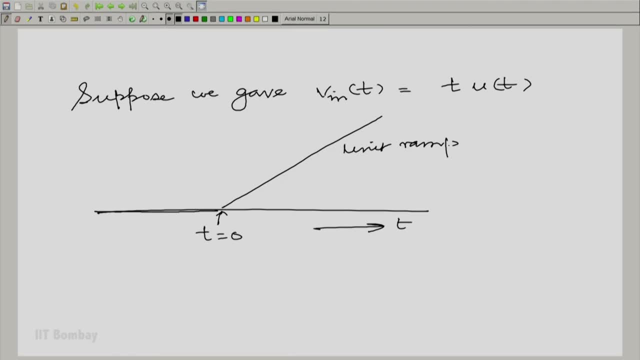 ever increasing. You will notice that the unit ramp is the running integral of the unit step, So it is equal to the integral from minus infinity to t? u lambda, d lambda and that amount. Then you have the way of leaving the kernel empty. Now you can solve this by two ways. One approach is: 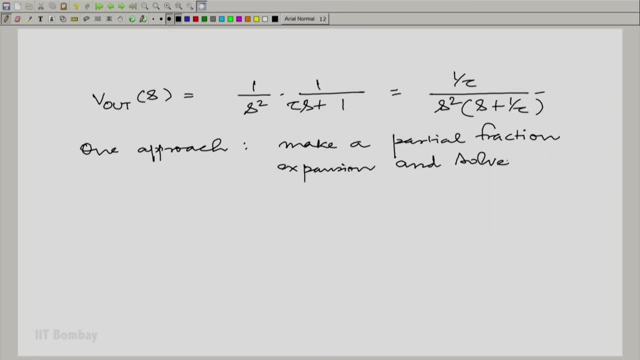 to make a partial fraction expansion. as usual. The second approach is to invoke the property of the linear shift invariant system. This operation of taking a running integral is itself a linear shift invariant system. So if you give it an input x of t and produce: 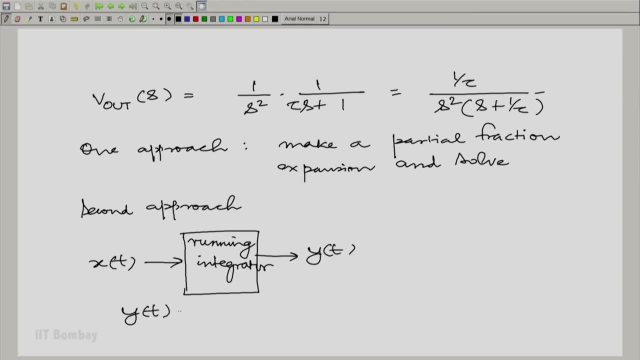 the output y of t, and if y of t is the integral from minus infinity to t, x lambda, d lambda, the system is linear, shift invariant and the system function is 1 by s. Now what you have done is to take the input unit step. you have given it to a running. 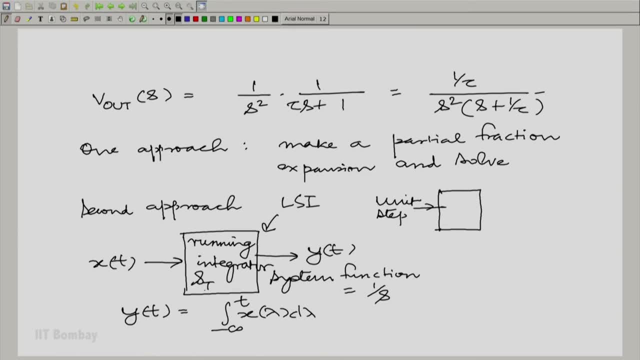 integrator. let us call it S i. let us call this system S i. you have given it to S i and you have given the output of this to the R C circuit. that is what you have done. Now this is a cascade of two L S i systems. We can interchange the order and therefore you. 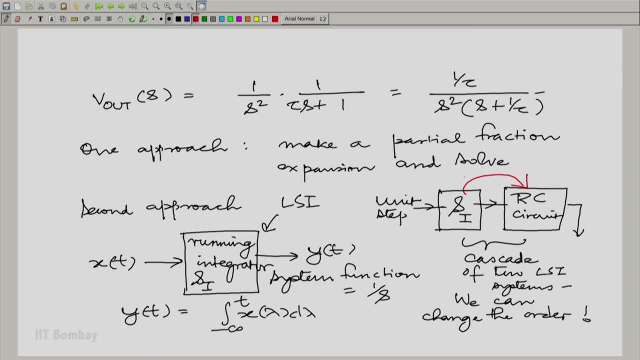 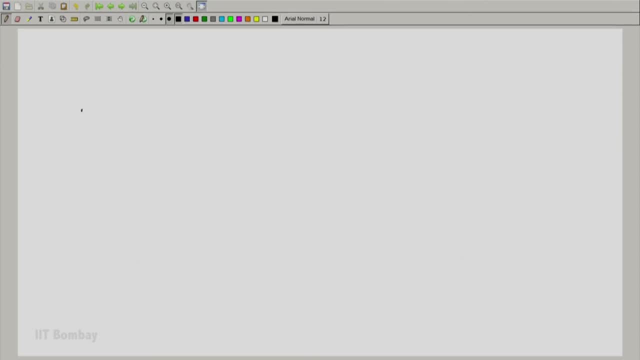 could put S i after the R C circuit, Which means you could have a situation as follows: you could give a unit step input, find the output to the R C circuit, which we already know, and this could be given to the.